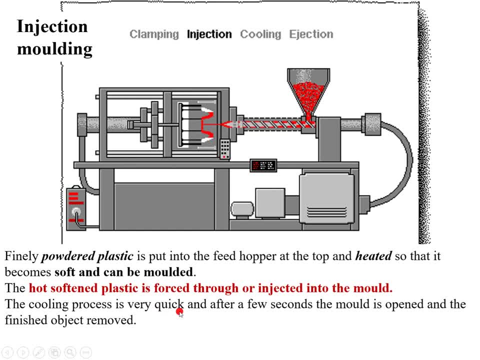 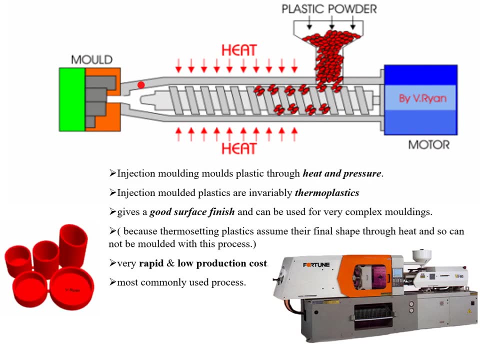 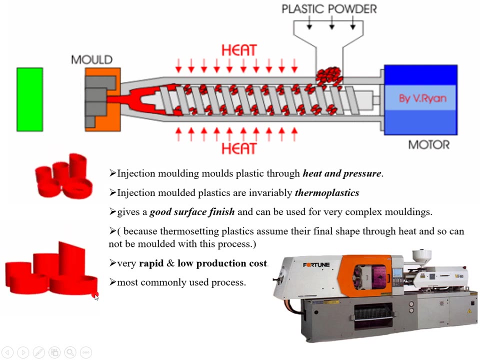 mold, Cool it. The cooling process is very quick And when you open the mold, the finished object comes out. The finished object can be removed. This is called as injection molding. Okay, And which types of plastic can be prepared? Now see, these are some of the key points that you can remember about injection molding. So injection molding plastic works on the 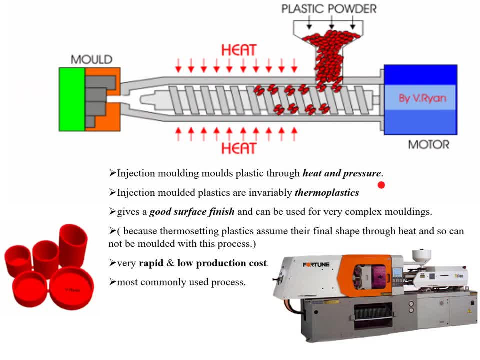 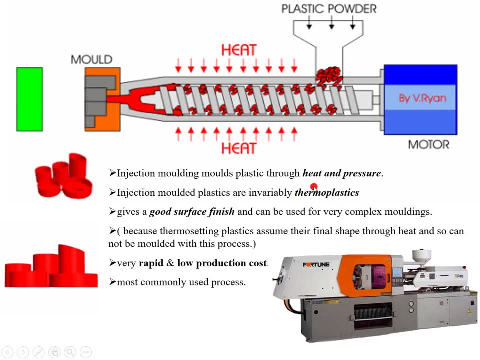 heat and pressure. Okay, That is how we are converting the powdered plastic into a softer one. Definitely, this is possible only for thermoplastic, because they can be softened on heating, and by applying pressure, Because of the process, you get a very good finishing for the plastic. Okay, Then this process is very rapid and has a low production cost, And this is the most commonly used process for a simple 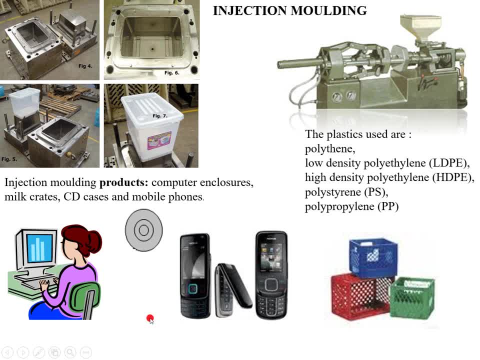 object Like these are some of the objects that can be prepared by injection molding: Milk crates, CD cases, mobile phones, These- all these are made up by injection molding. See, this is a product Basket. This is a final product of the injection molding, So you can see the molds, how the molds are, depending on what shape you want. You can prepare those molds And all thermoplastics can be used, For example, LDP, polythene, LDP, HDPE are different. 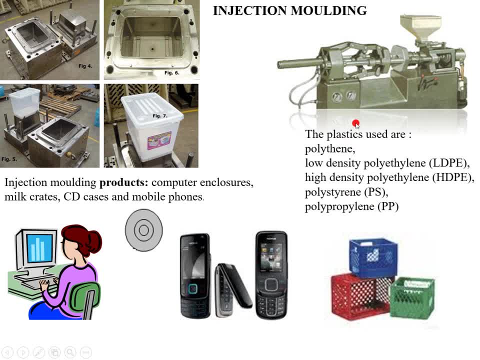 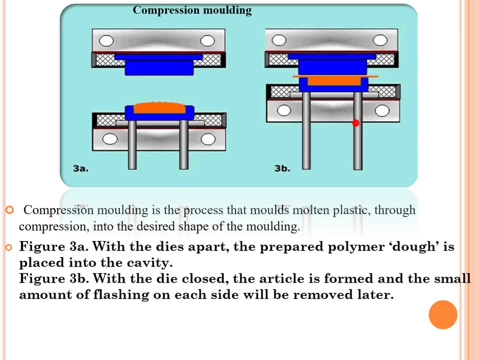 different types of polythene, polystyrene, polypropylene. all these are thermoplastic polymers which can be molded by injection molding. The next method is compression molding. Look at this image over here. This is the plastic that we have taken in a mold and we 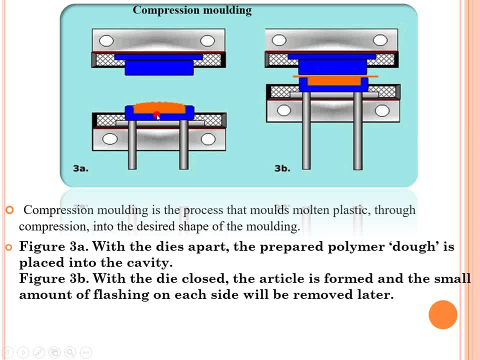 just apply pressure from the top. So whatever is the shape of the mold will be acquired by the plastic. Okay, So compression molding is a process that holds molten plastic through compression into the desired shape of molding. So this is the dough, This thing that we 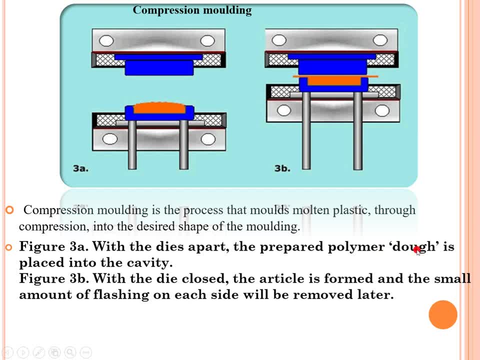 take as a plastic, soft plastic. this is called as a dough. It is a polymer dough which is placed in the cavity. and these are the two dyes. This is the upper dye, this is the lower dye, and then you just compress it, you just press it and you get this. 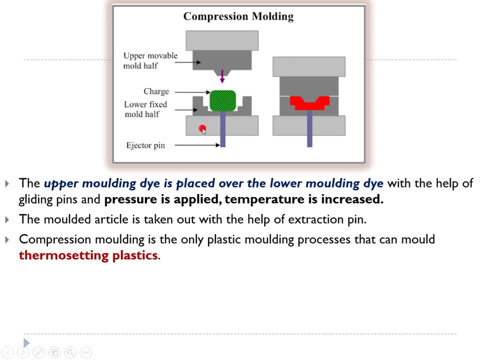 And then you just press it and you get the desired shape. Because of this type of process, this type of process- you can see this is used for thermosetting plastics. right? You cannot use injection molding for thermosetting. So if you want to mold a thermosetting plastic, 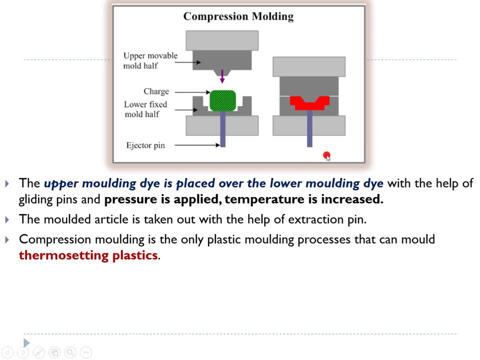 like bake light. Okay, So for that we can use compression molding. So upper molding dye is placed above the lower molding dye with the help of gliding pin. So for that we can use compression molding. So this is the process which we have taken to mold the 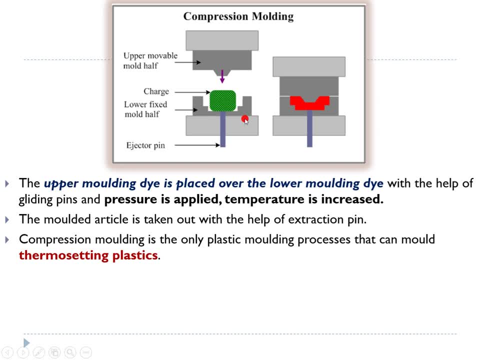 plastic. So if you want to use injection molding, we can just press it and you can place it. pressure is applied, temperature is increased, it will become, the temperature is increased and this process takes place. so it's quite easy to understand this. okay, so these are some of the products which are made by compression. 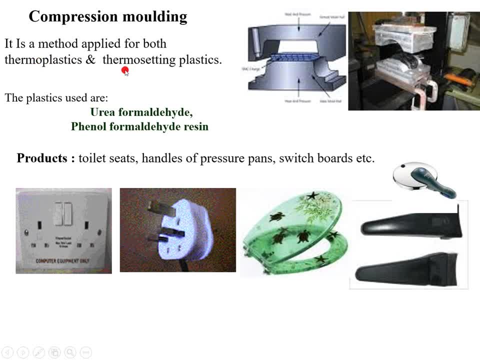 molding. of course it can be applicable to plastic, see thermoset. if it can mold thermosetting plastic, it can thermosetting. it can, of course, mold thermoplastic. okay, what are the plastics used? urea, formaldehyde, phenol, formaldehyde, bakelite- that's bakelite. so these are some of the objects. 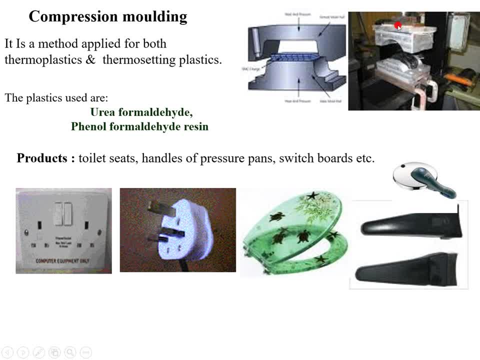 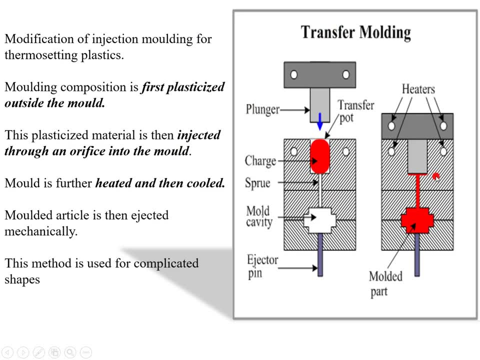 that can be prepared by compression molding. this is the actual compression molding. okay, let's go to the next one: transfer molding. just look at the diagram over here. okay, so this is the upper part. this is the mold cavity. it will. it depends upon the shape of the plastic that you want. this is a modification of injection. 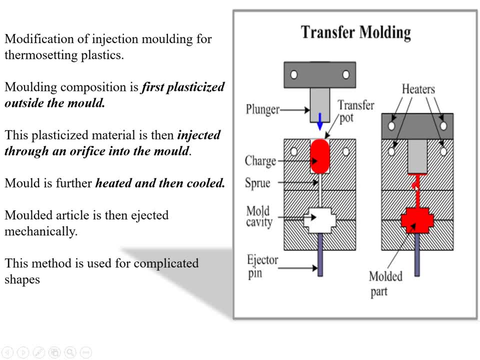 molding, kind of injection molding, so you can see there is a screw from which the plastic can go into the mold. so what are the steps in molding? the plastic is first made softer, it the plasticized. the plastic is made softer outside- okay- and then it is placed in the mold. so this is the plastic, softened plastic- then. 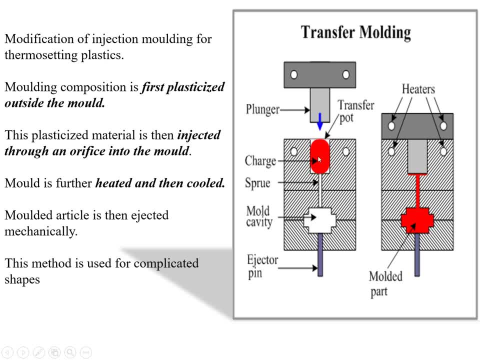 through pressure. this plastic is injected through the orifice into the mold. in the mold you have this heating and cooling taking place. so once the shape is formed, it is cooled and the molded article is ejected mechanically. this type of process is used for preparing complicated shapes of 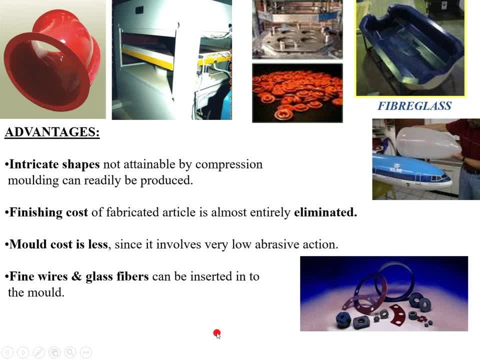 plastic. these are some of the examples. okay, these are some of the objects which are prepared by transfer molding, so intricate shapes which cannot be made by compression molding can be produced. finishing cost is eliminated because you get a very good finished product. mold cost is less. okay, fine, 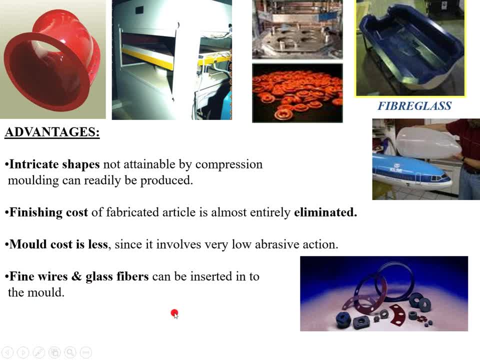 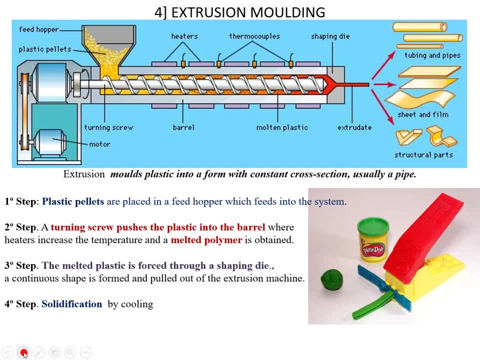 wires, glass fibers can be inserted into this mold, depending upon what, what type of shape or plastic you are preparing for. and the last one is extrusion molding- extrusion, so it is similar to injection molding. the only thing is the plastic part that is coming out. it is removed it. 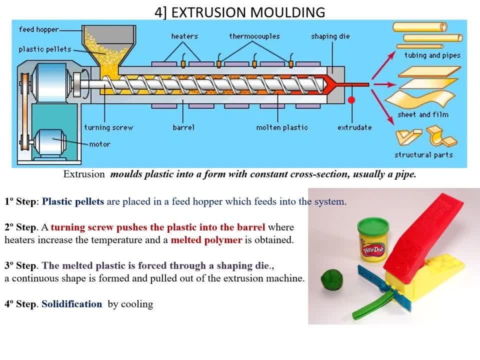 is excruated, okay, and that is how you get these typical shapes. pipes can be made, sheets or films can be made by extrusion molding. so the process is similar to injection molding. you take the plastic pellets, mix all the ingredients and everything, take the plastic pellets. 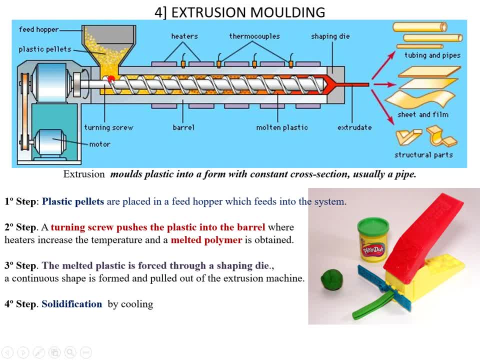 fill it in the hopper, okay, then through the hopper it goes into the barrel. there is heating, heating taking place, so it softens over here, fine, and the plastic is pushed. the softened plastic is pushed outside and here at the outlet there is a shaping die. so the melted plastic is close to the shaping die and the shape. 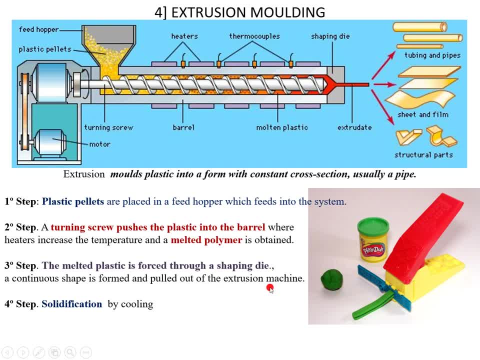 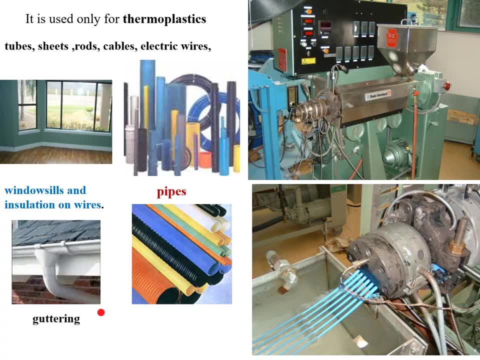 is excluded outside. it is pulled outside through an extrusion machine and then, of course, once you get the mold, you pull it and you have your product. okay, so these are some of the shapes that we can get by extrusion molding. this is the actual extrusion moulding machine, so this can be used, of course, for 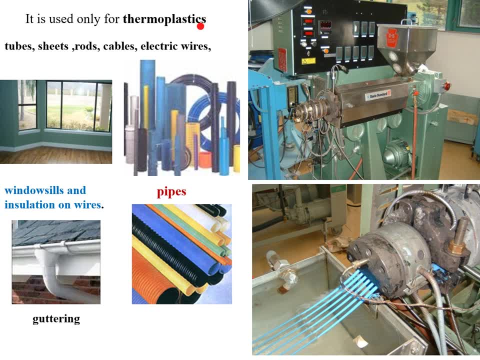 thermoplastic, because you have to melt, not melt as much, you have to make the plastic soft. so tubes, sheets, rods, cables, all these are prepared by extrusion moldingçe. okay, let me take it. so this is extrusion molding, so you need to how many thin pieces you want, or huh, how type size. so this is an extra. 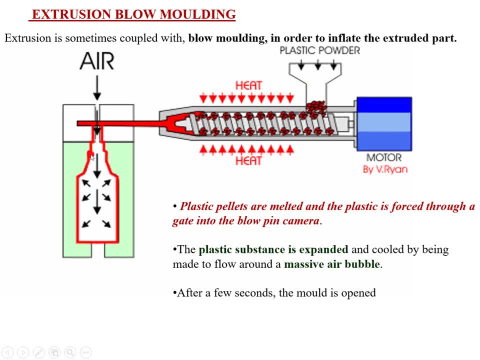 having in the cool in this molding, okay. okay, now into the next. this is a left hi two feet carriage, detta. now all right here, Karena, came to you from back in the. This is extrusion mold molding, exclusively used for preparing shapes like bottles. Okay, So, once the plastic is extruded, blow some air into it, prepare a mold, separate mold over here, So the extruded part is inflated.